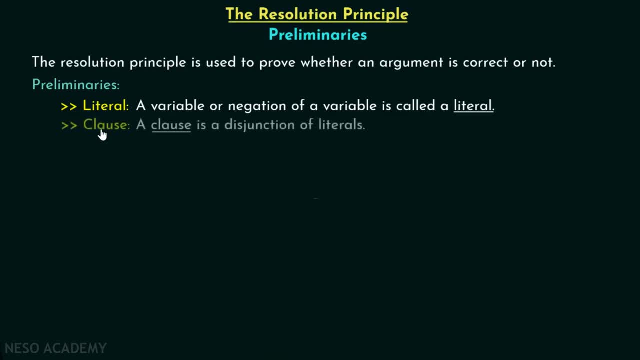 a literal Fine. Now there is one more term, which is called clause, and we must understand what this term is. A clause is a disjunction of literals. Okay, You take some set of literals and form the summation of them. The results obtained is called a clause Fine. And there is one more term that 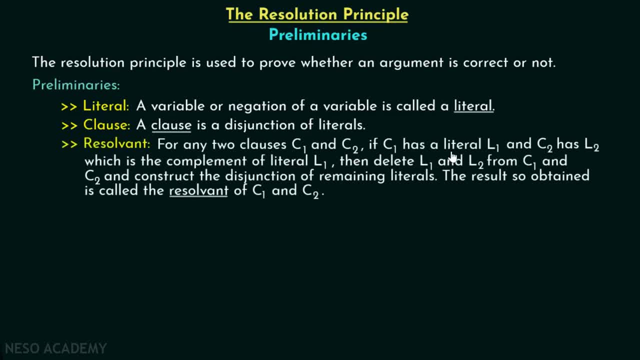 is called resolvent For any two clauses c1 and c2,. if c1 has literal l1 and c2 has l2, which is the complement of literal l1,, then delete l1 and l2 from c1 and c2.. Here we have two clauses, c1 and 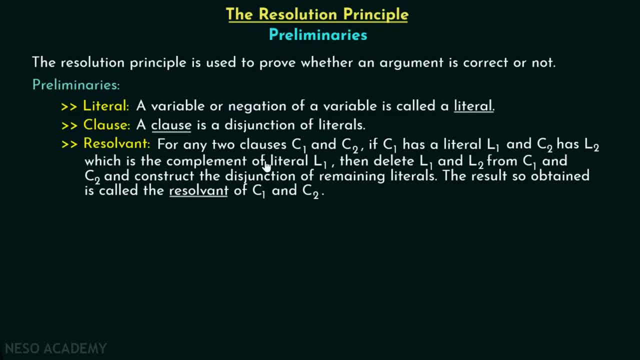 c2.. c1 has literal l1 and c2 has literal l2, which is the complement of literal l1.. Right, We have c1 and l2 in c2.. l1 and l2 are complementary to each other. Our job is to delete l1 and l2 from c1. 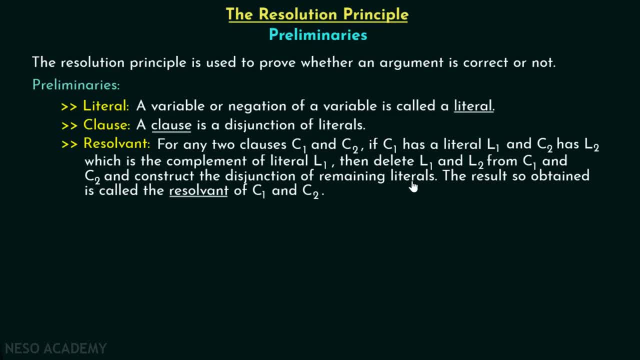 and c2, and we will construct the disjunction of remaining literals. The result so obtained is called the resolvent of c1 and c2.. Okay, We will understand this with the help of an example. Let us suppose that c1 is p or q or r and c2 is not p or s or t. These are two clauses. Right, We can. 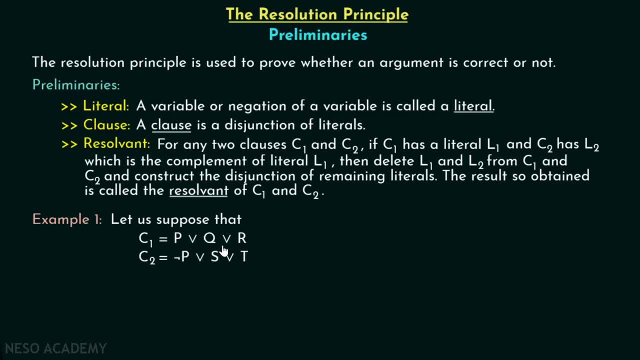 see that p, q, r and we are forming the disjunction of these literals. So this is a clause and this is also a clause Here. instead of p, we have not p and we have s and t over here. These are two. 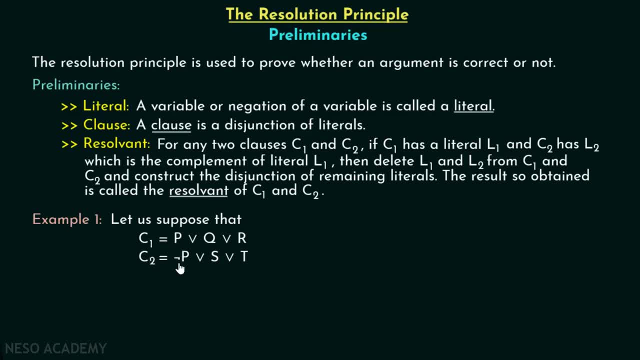 clauses: Right, You can see that here we have p and here we have not p. p and not p are complementary to each other. They are like l1 and l2.. Right, p and not p are complementary to each other According to the definition of resolvent. delete p and not p and take the disjunction of the. 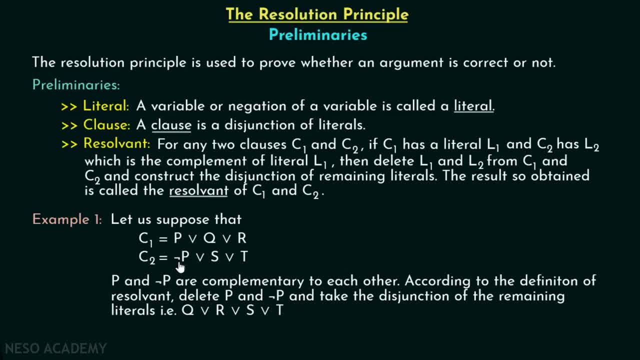 literals. We will first delete this p and not p. Then we are left with q, r, s and t. We will take the disjunction of these remaining literals, That is, q or r or s or t. q or r or s or t. This 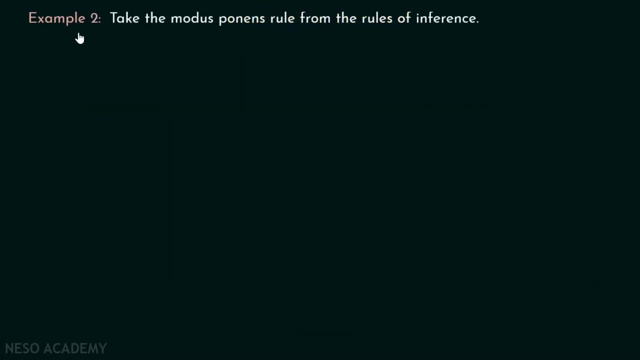 is the result so obtained and this is called resolvent. Now let us discuss example 2.. Take the modus ponens rules from the rules of inference. So this is modus ponens rule p and p implies. q implies q. We can write this as p and p implies q. We can write this as p and p implies q. We can. 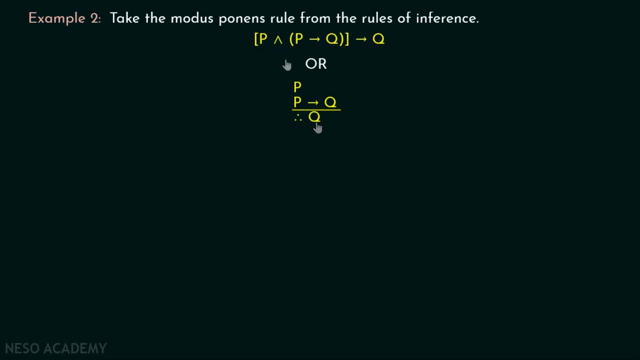 write this in this form as well: p, p implies q, therefore q Whenever you find, and in between you can divide them. You can first write p and then you can write p implies q, Then you can write q. This is the conclusion, Right? In order to find the resolvent from the premises, we will. 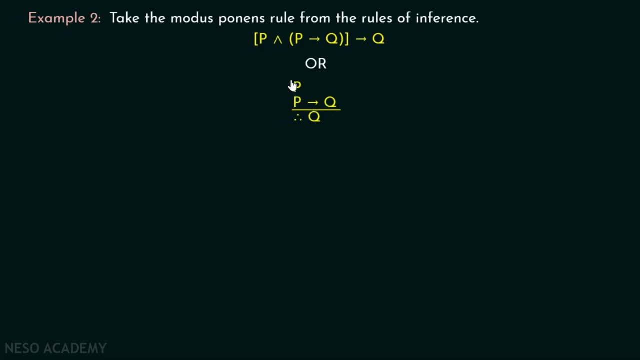 write the clause form of p implies q. Okay, p is fine, This is a literal, But p implies q is not in a clause form. So we will first write the clause form of p implies q. We know that p implies q is equivalent to not p or q, And this is in clause form. Right, We have this literal and this. 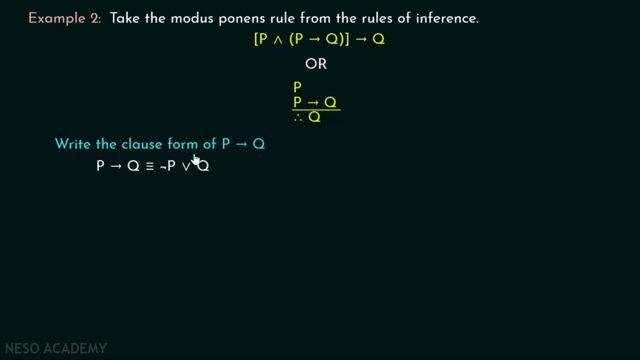 is not p And we have taken the disjunction of these two literals. So this is nothing but a clause form. So first clause is p and second clause is not p or q. So c1 is p and c2 is not. 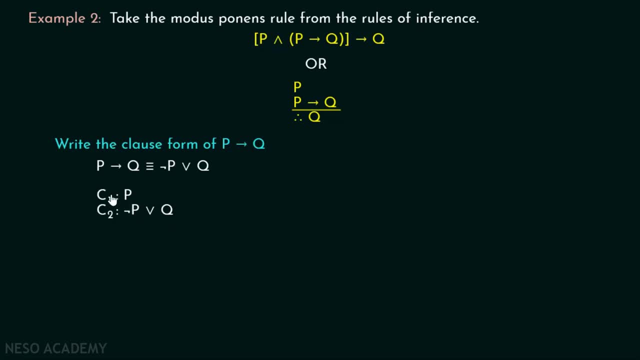 p or q. From these two clauses we can easily find the resolvent. First we have to delete p and not p Right, Because these two are complementary to each other, And then we will take the disjunction of the remaining literals. You can see over here that we are left with just one literal Right. So 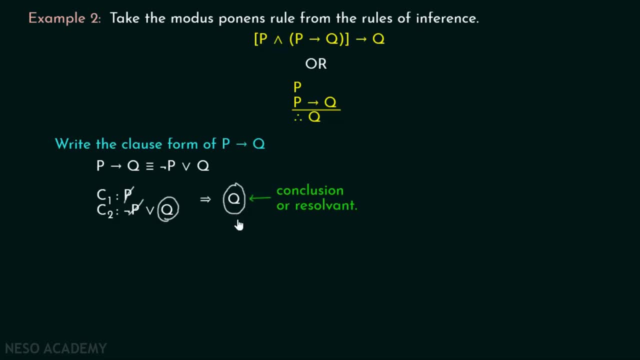 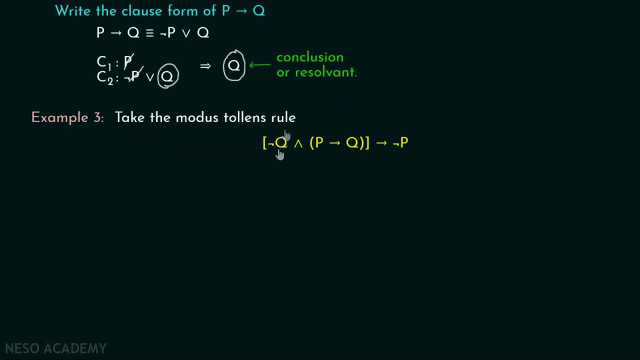 this is the conclusion, Isn't that so? And this is the resolvent as well. This is nothing but a conclusion, as well as the resolvent. Let's discuss one more example. Take the modus tollens rule, Not q, and p implies. q implies not p. This is modus tollens rule. We can write: 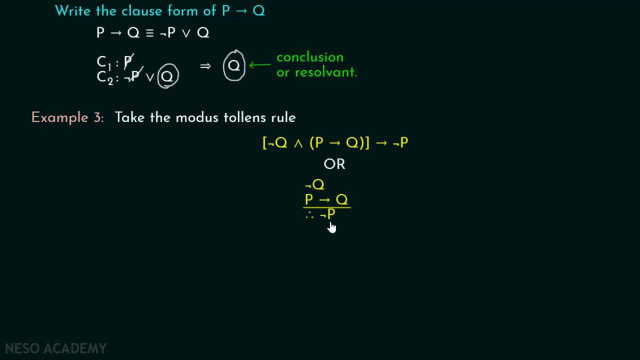 this in this form as well, Not q. p implies q, therefore not p. First we will obtain the clause form of p implies q. We know that clause form of p implies q is nothing but not p or q. So c1 clause is not q and c2 clause is not p or q. We will try to find the resolvent from these. 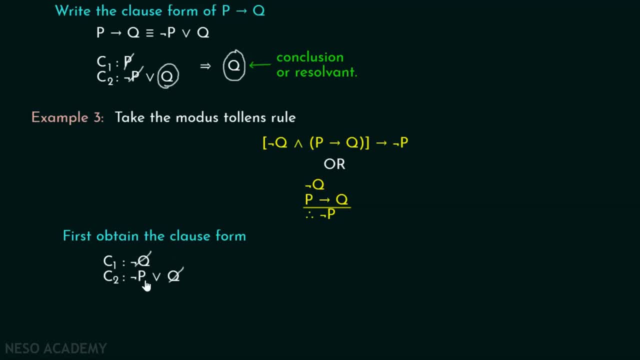 two premises. We will delete not q and q, and the remaining literal will be not p. So this is the resolvent And let me tell you this is the conclusion as well. You can see that we have obtained not p as a conclusion from these two premises. So there is one theorem which actually 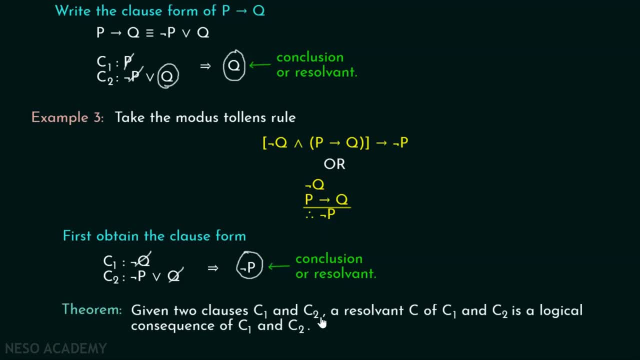 is the base of this argument. Given two clauses- c1 and c2, a resolvent c of c1 and c2 is a logical consequence of c1 and c2.. That is what we have seen Right: The resolvent solution of c1 and c2.